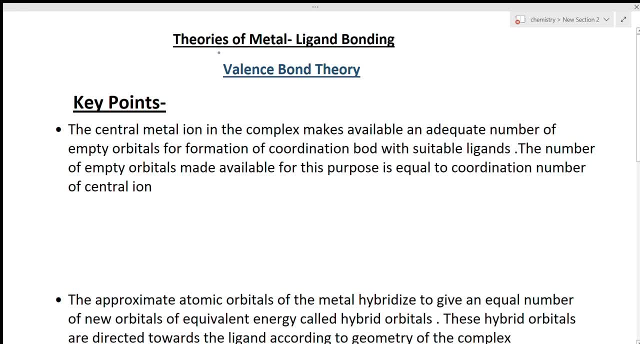 Now we are going to start the theories of metal ligand bonding. There are some theories related to metal ligand bonding. The first of these is valence bond theory. Okay, that is also called VBT. Okay, so valence bond theory, which was first given by Pauling. 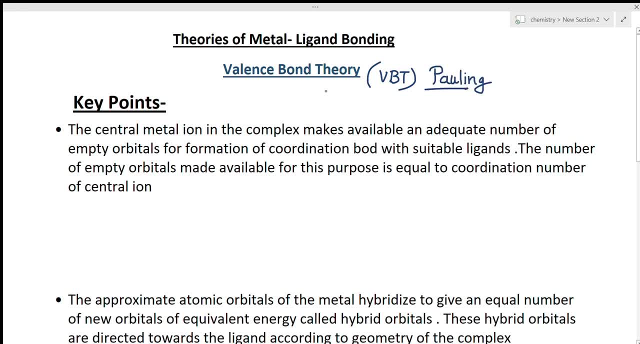 Okay, after this all the other theories came. So that is why we will first read valence bond theory. So key points. what were some key points of valence bond theory? The central metal ion in the complex makes available an adequate number of empty orbitals for formation of coordination bond. 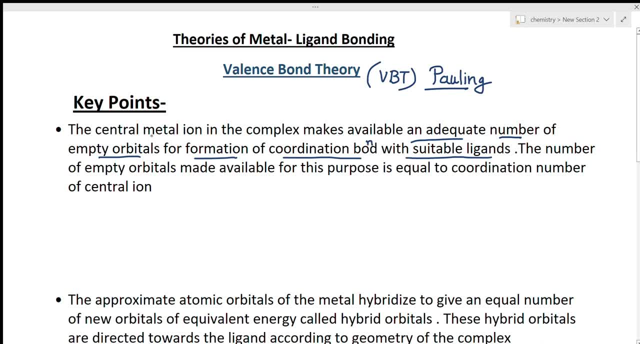 Coordination bond with the suitable ligands. Okay, So what does the central metal ion do? To make coordination bonds with all the ligands, an adequate number of empty orbitals is made available. Okay, The number of empty orbitals made available for this purpose is equal to the coordination number of central metal ion. 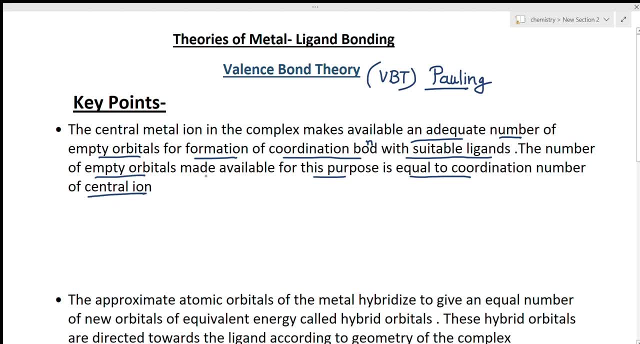 So all the orbitals, all the empty orbitals will be made available. Their number actually is the coordination number of the central metal ion. So the coordination number of the central metal ion is equal to the coordination number of the central metal ion. 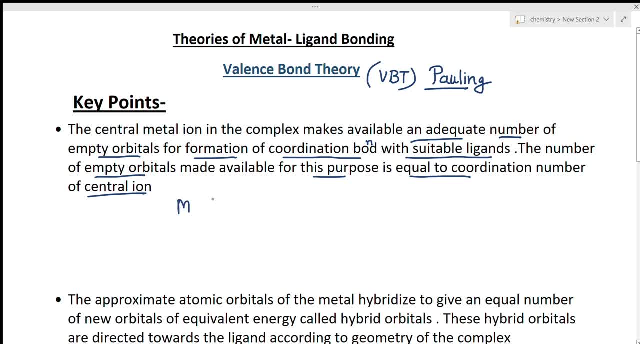 Suppose you have taken any metal M which is making octahedral complex. Okay, If our metal is making octahedral complex, it means what is happening in it? There will be due to hybridization through sp. Why will it happen? 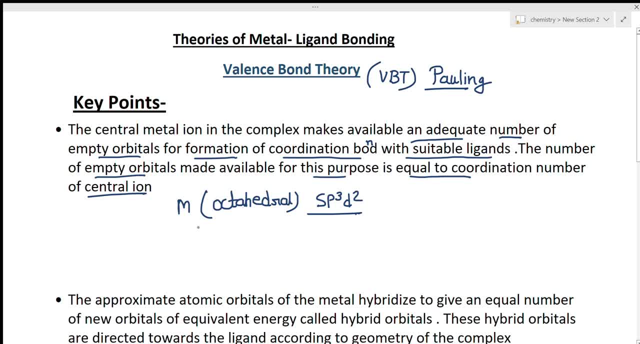 Because here, whenever octahedral complex will be made, then how many ligands will be separated from metal? Six ligands, Okay. So to accommodate the electron pairs of six ligands, six orbitals will be required. Six vacant orbitals are needed. 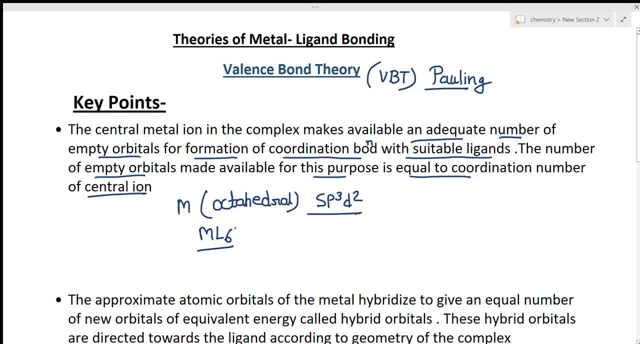 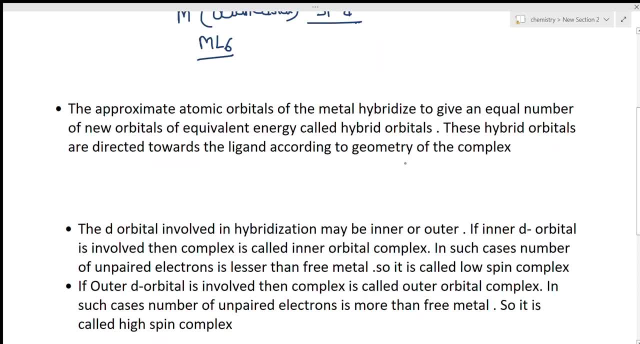 So these six vacant orbitals will need empty orbitals. So what type of hybridization will happen here? There will be sp3d2 hybridization. Okay, What is the second point? The approximate atomic orbitals of metal hybridized to give an equal number of new orbitals of equivalent energy, called hybrid orbitals. 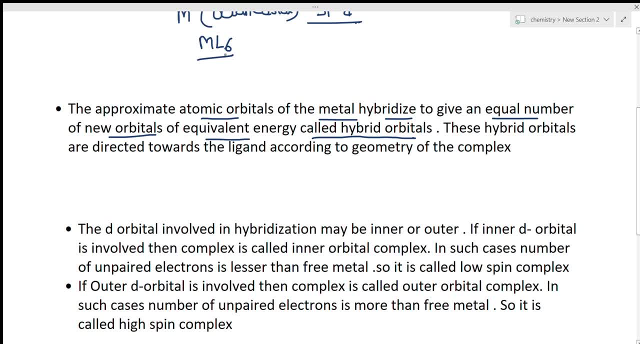 Which I just told you. Whenever ML6 type of complex is made, it means six hybrid orbitals are needed. Six orbitals are needed. Okay, Six empty orbitals are needed. Now these orbitals? suppose you took sp. 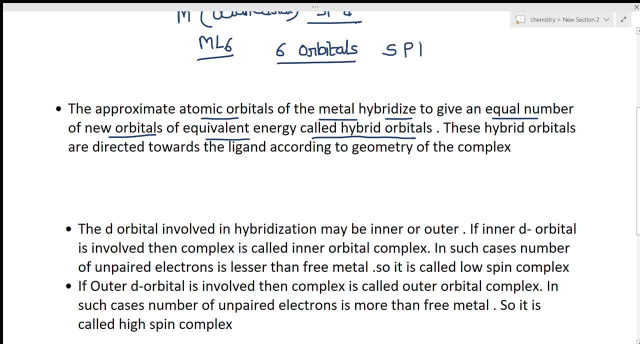 took 3p orbitals, or you took 2d orbitals. What are the energies of all these? They are different. Whatever orbitals, we need the geometry of all of them, the energy of all of them, the shape of all of them. 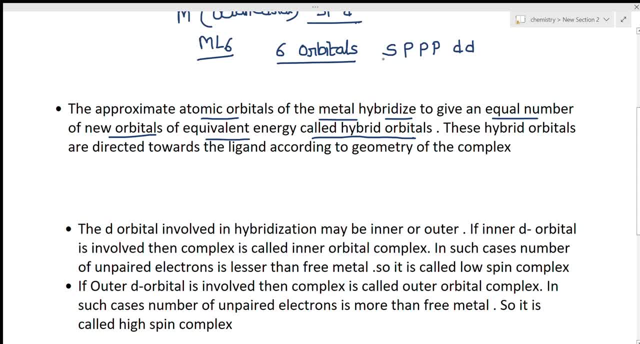 should be equivalent. So what will happen for this? There will be hybridization between them. Okay. So what is happening here? There will be hybridization, Okay. So what is happening here? There will be hybridization, Okay. 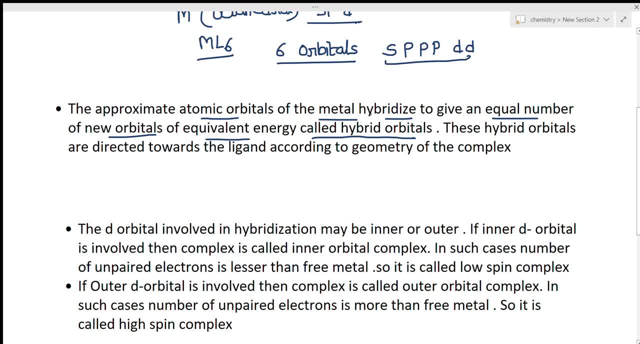 So all these approximate orbitals, all these metals we had, what happens between them? hybridization takes place and new hybrid orbitals are made whose energies are the same. These hybrid orbitals are directed towards the ligand according to the geometry of. 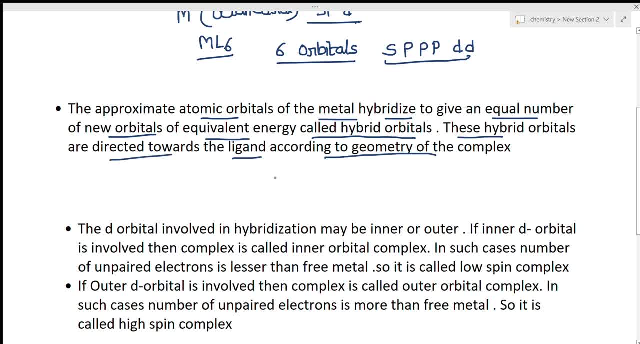 the complex. Now, these hybrid orbitals which will be made, like these sp3d2 hybrid orbitals will be made. So what will happen? All of the metals, all of these hybrid orbitals will be directed towards the ligand. 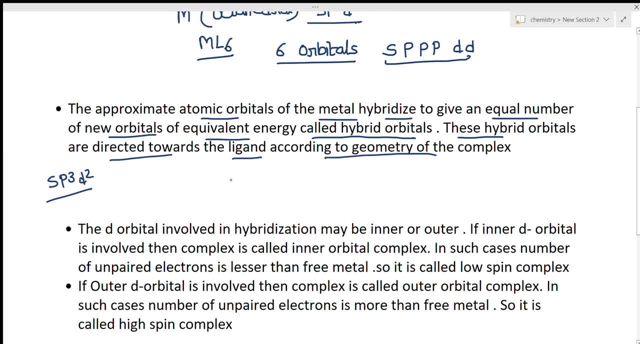 according to the geometry, which means if its geometry is octahedral, it is metal. then it will be oriented to our ligands from this type. The next point says that the d orbitals involved in the hybridization may be inner or outer. 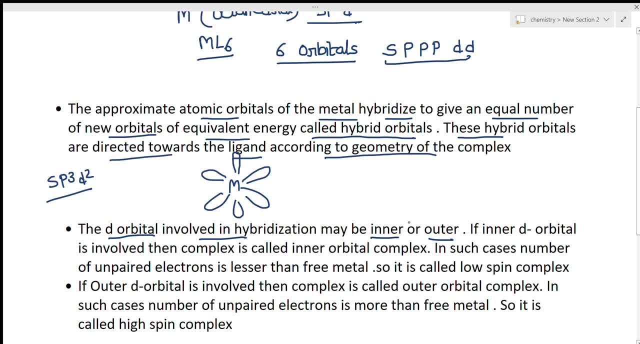 The d orbital involved in the hybridization can either be inner or outer. Inner means n-1d, or it can be a penultimate d shell, or it can be nd, ie outer d shell. If inner d orbital is involved, then the complex is called inner orbital complex. 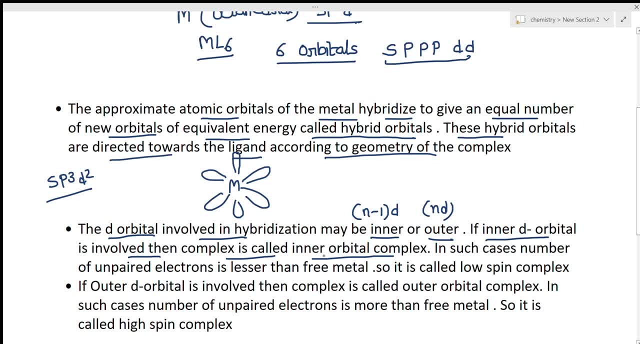 If inner d orbital is involved, then we call such complexes as inner orbital complexes. In such cases, number of unpaired electrons is lesser than the free metal. What happens in such cases? The number of unpaired electrons in the complex is lesser than the free metal. 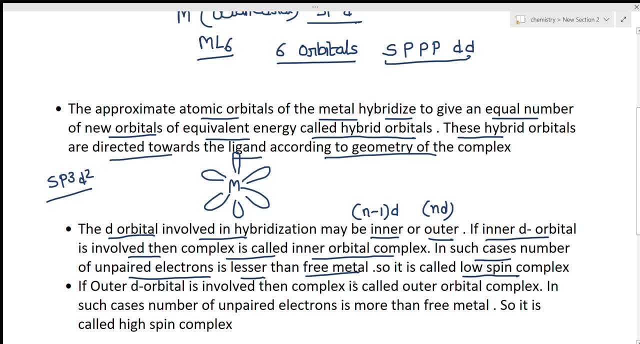 Such complexes are known as low spin complexes. When you look at the examples, you will understand how low spin complexes are. If outer d orbital is involved, then the complex is known as outer orbital complex. Such complexes are known as outer orbital complexes. 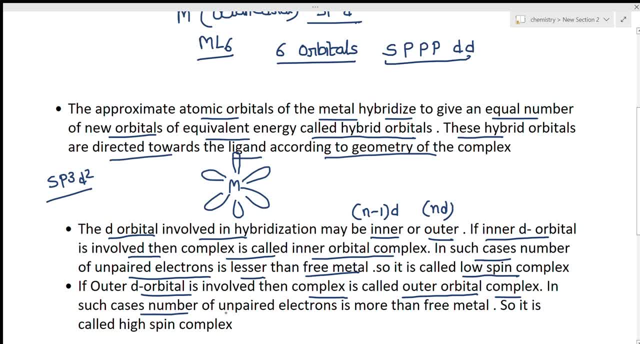 Such complexes are known as outer orbital complexes. In such cases, the number of unpaired electrons is more than the free metal. In such cases, the number of unpaired electrons is more than the free metal, So it is called high spin complexes. 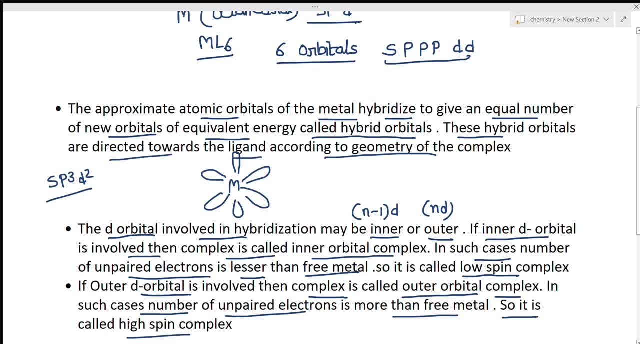 So such complexes are known as high spin complexes. So high spin complexes and spin free complexes are the same. These complexes are known as high spin complexes and spin free complexes. Now we will understand this with the help of examples. Okay, 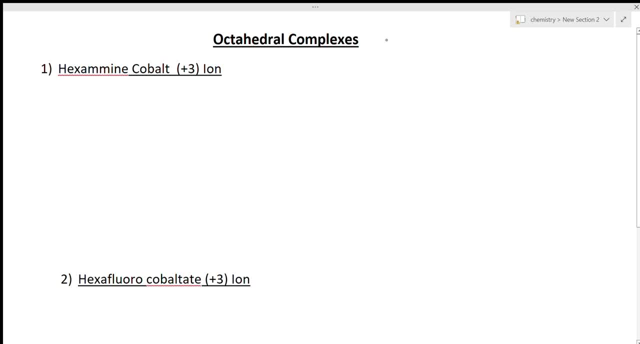 So the first example we will see is of octahedral complexes. How do we make an octahedral complex? The first example is of hexamine cobalt, third ion. How do we write down hexamine cobalt, third ion, CO, N3, whole six plus three? 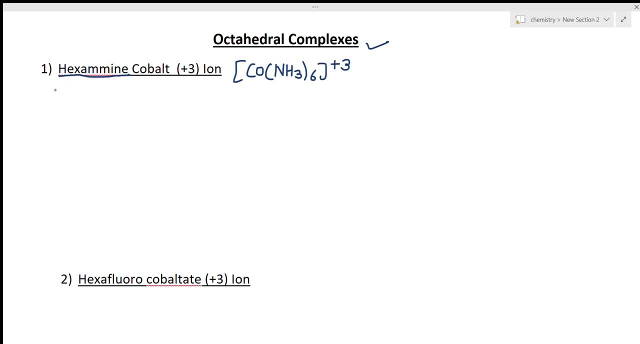 Okay, If you look at this, complex cobalt is present here in the plus three oxidation state. When you look at cobalt in the plus three oxidation state, then how does this happen? There is a configuration of 3D6.. Okay. 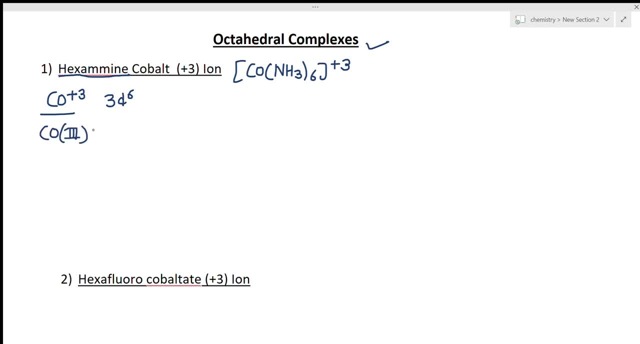 There is 3D6.. So first we will see cobalt, third Cobalt, third, 3D6.. That means we have made this as orbital. Okay, Now see, there are six electrons here: One, two, three, four, five and six. 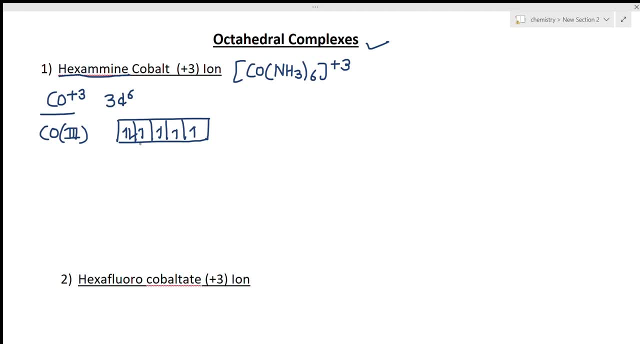 What is this? This is the free state of metal, Whereas metal has six electrons present in the d orbital. Okay, This is your s orbital and this is your p orbital. What will we call this d orbital that is involved n minus 1 d orbital. 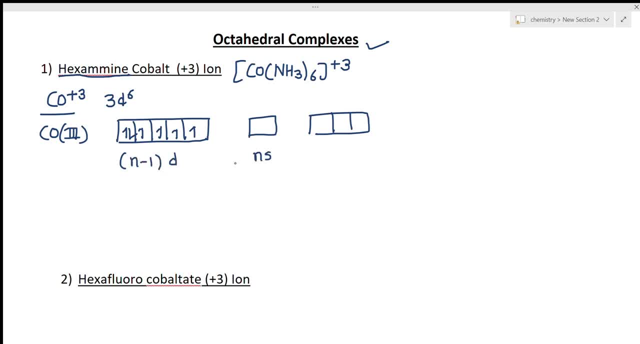 This is inner d orbital, This is our ns orbital, This is outer s orbital and this is our np orbital. Okay, This is 4s, this is 4p and this is 3d orbital. That means this is inner d orbital. 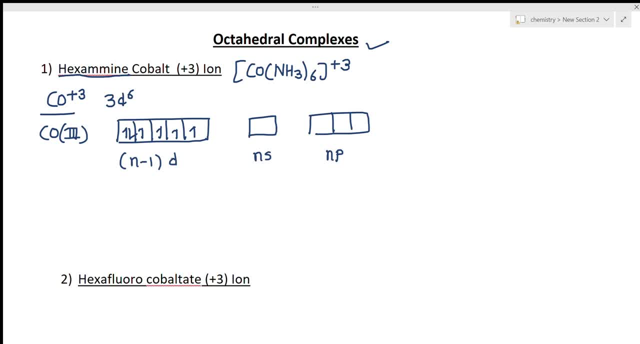 This is being involved. That is why we will call these complexes inner orbital complexes. How is it being involved? See Now what will happen. You have seen this free state Here. when you were looking at the free state, then all of them. 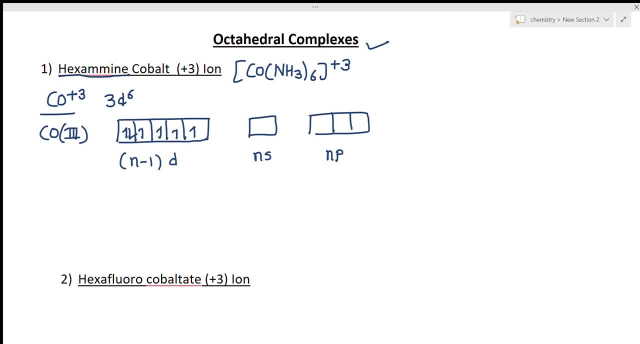 all of the d orbitals were filled. Okay, Here there were two electrons, Rest of them were of one electron. Okay, Now the first line that you had read. What was the first point? That metal makes available empty orbitals. 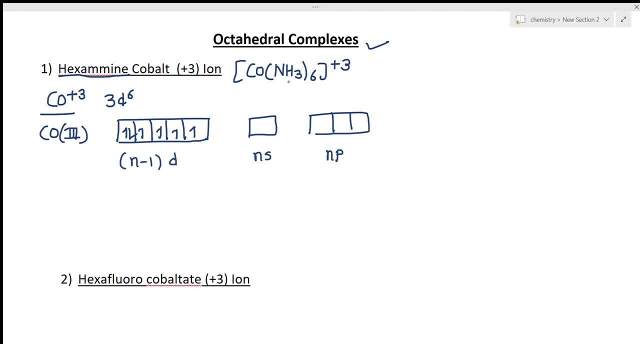 As according to the number of the ligands. Okay, Metal, according to the number of these ligands, makes available all the orbitals that are needed. Okay, So here you are, seeing that six orbitals are needed Because there are six ns3 ligands. 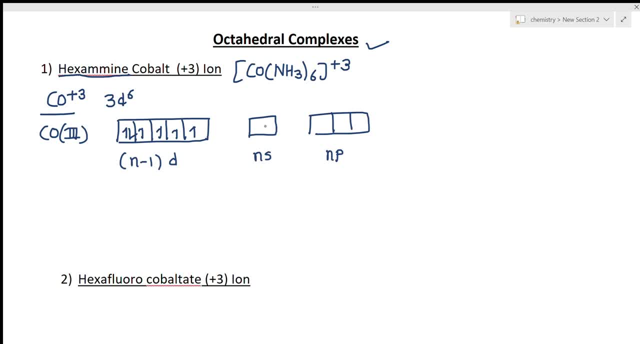 Here there are six ammonia ligands: One, two, three and four. These four orbitals are present here. Okay, If these electrons are paired up, then two more orbitals will be available here, And actually this happens. 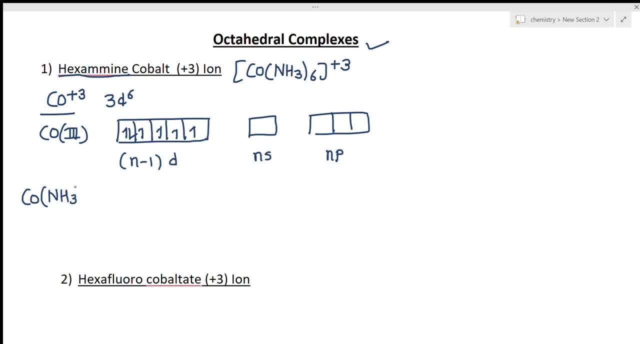 Why does it happen? Because CO ns3- whole six plus three complex ammonia ligand is present here And it is sufficiently strong to pair these electrons. So what does it do? It pairs these electrons. So what happens? These electrons? 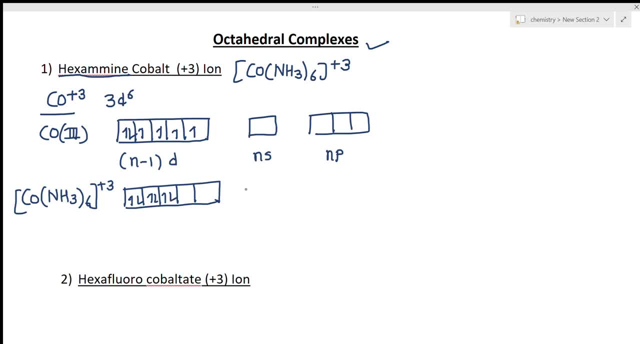 where did these electrons come Here? Now see this: Two d orbitals are available here. One is s orbital and the other is 3p. That means you needed six empty orbitals in total, And six orbitals are available here. 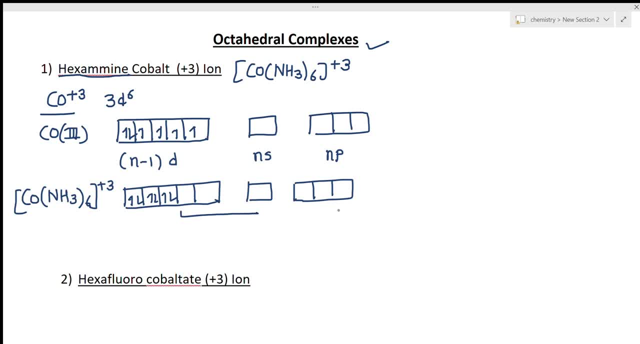 Okay, Now the hybridization that will happen between them. that is called sp3- d2.. Now see this: You have taken inner d orbital, So what will we write for it? d2- sp3 hybridization. What will we call this type of complex? 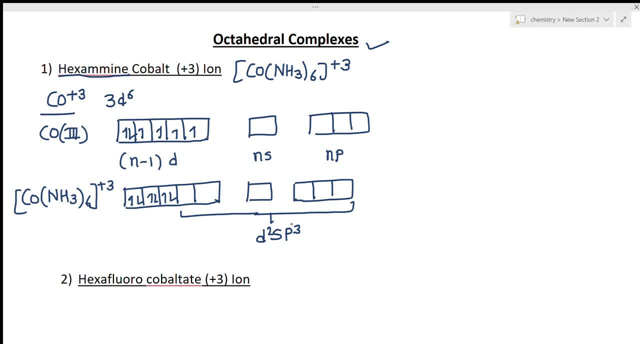 Inner orbital complex Because inner orbital is involved. Okay, Now six hybrid orbitals are formed. These hybrid orbitals will be octahedrally oriented towards ns3 ligands. Okay, Now see, what will six ns3 ligands do? 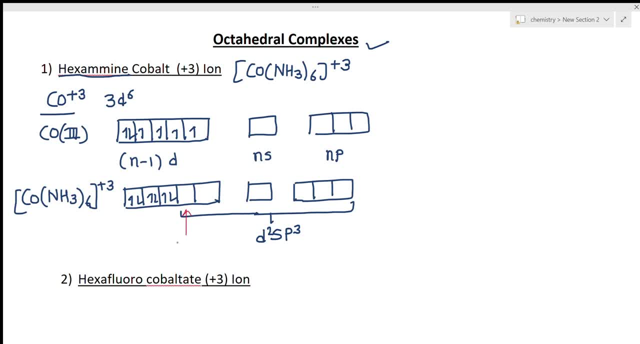 They will accommodate electrons in them. These are your ns3 ligands And we are showing their electrons from cross. Okay, These are their electrons. Okay, We can identify them with this. That is why we are showing them from cross. So these electrons will be accommodated in these d2 sp3 hybrid orbitals. 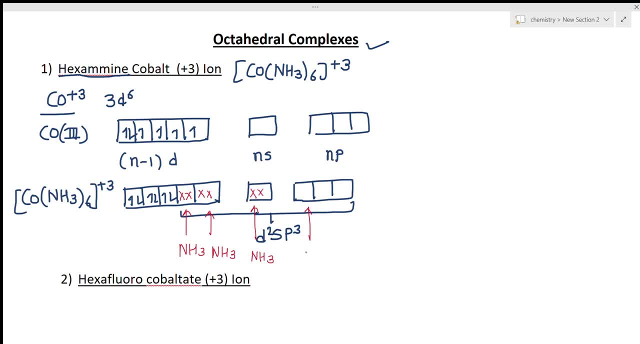 These d2- sp3 hybrid orbitals will be octahedrally oriented towards these ns3 ligands. Okay, Here the orbitals of these ligands and the orbitals of these ns3.. Okay, The orbitals of the ligand and the orbitals of the d2- sp3 hybrid orbitals of the metal. 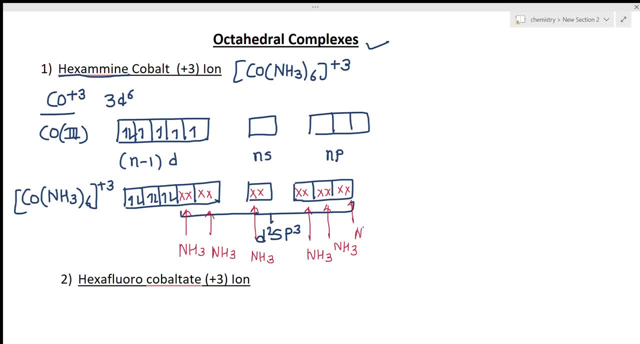 what will happen here? It will be overlapping And in this way, the electrons from ns3, they will be donated here. So here you can see how all the electrons are paired. Okay, All the electrons are paired here. So how will we call these types of complexes? 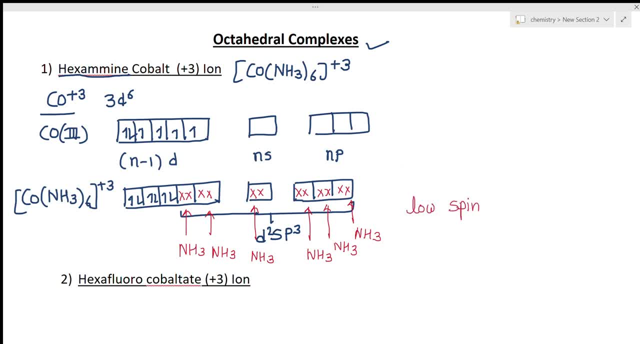 We will call them low spin complexes. What did you see here? There were four unpaired electrons in the metal. Okay, Here four unpaired electrons were present. Okay, One, two, three and four. But when your complex was made, 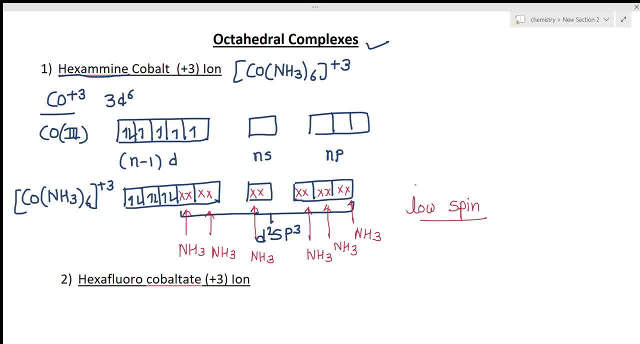 there were not even eight unpaired electrons in it. So whenever the number of unpaired electrons in the complex is less as compared to free metal, then what do we call such complexes? We call them low spin complexes. Okay, Now let's see the next example. 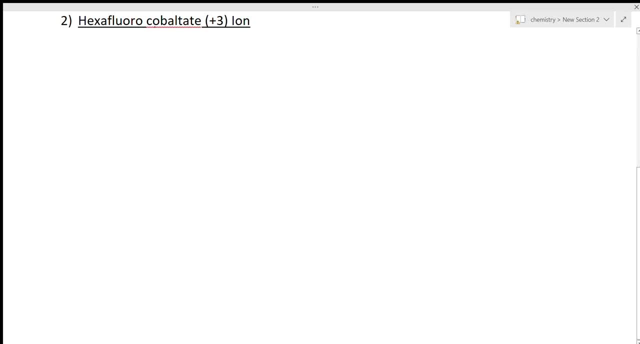 Next, your example is hexafluoro cobaltate plus 3 ion. How will we identify this? COF6 minus 3.. Okay, Now, here also, you see the cobalt plus 3 oxidation. That means again, this is your D6 configuration. 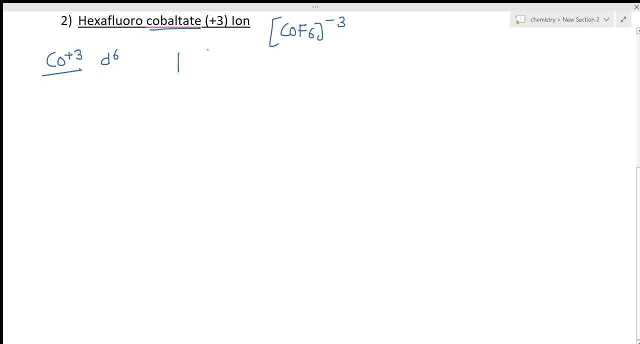 Okay. So when you make this, how will it look like when you are looking at it in free metal? One, two, three, four and five? The orbitals are here. Okay, Now let me show you where this outer D orbital is. 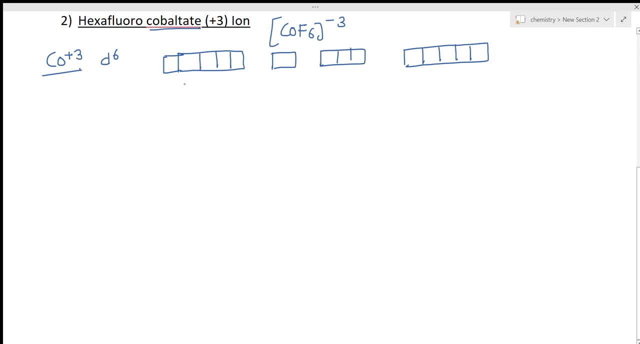 This is the outer D orbital. This was your N minus 1, that is 3D orbital. This was your 4S orbital. This is 4P orbital And this is your 4D orbital. Okay, So how many electrons were present here? 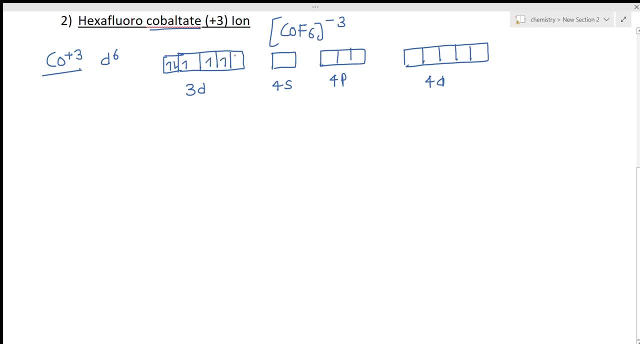 One, two, three, four, five and six orbitals. So here six electrons were present. Okay, Total there were six electrons. Now how many electrons are there? Look how many orbitals are needed. Here COF6 is being formed. 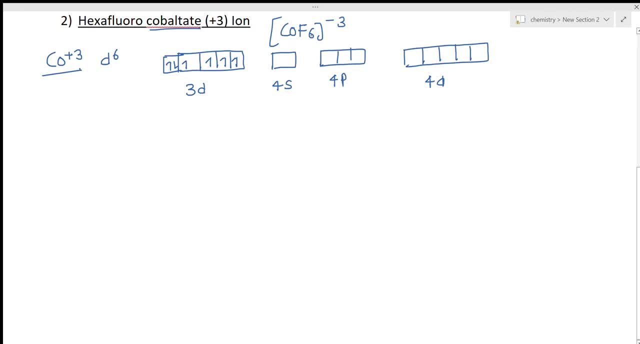 COF6 means 6 fluorine ligands are attached here. When 6 fluorine ligands are attached, then it needs 6 hybrid orbitals. That means it needs 6 empty orbitals. So what will happen, What should happen here again? 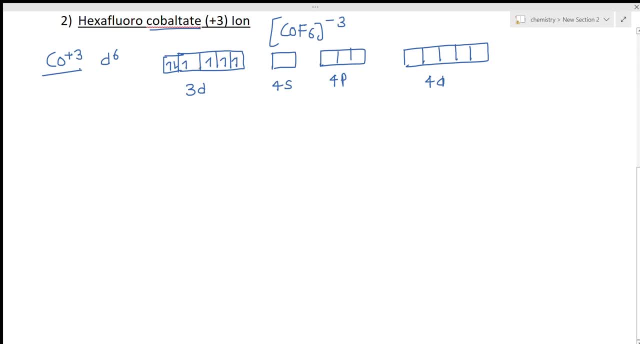 There should be pairing. Can we pair electrons? No, we cannot do this. We cannot do pairing here. If you see COF6 minus 3.. So the ligand which is present here is actually a fluorine ligand. 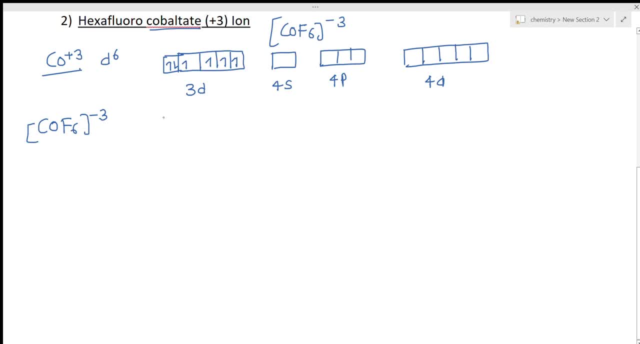 And fluorine ligand is a weak field ligand. Okay, So whenever there is a weak field ligand, it does not take the pairing of the electrons, So these electrons will remain as it is present. Then what will happen? 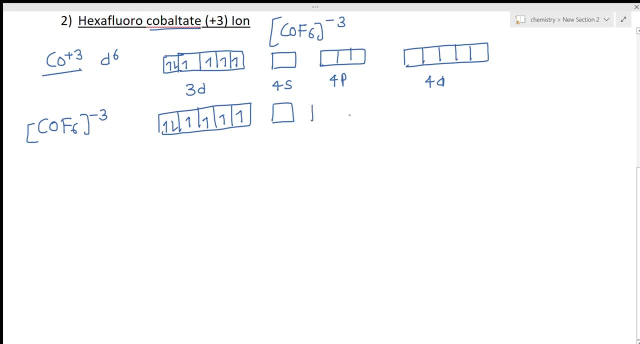 Then the condition will be that these s orbitals, these 3p orbitals and these 2d orbitals will do hybridization. Now, what will we call the hybridization that is happening? What will we call it SP3D2 hybridization? 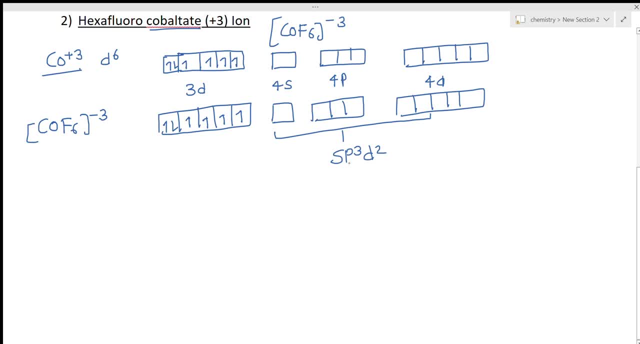 Due to this sp3d2 hybridization, 6 new hydrid orbitals will be formed which will be octahedrally oriented, That is, they will be oriented towards ligands. Now, what will your fluorine ligand do? 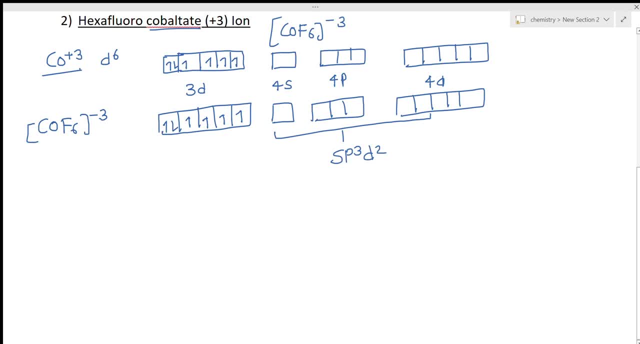 It will donate a lone pair of electrons. What did we read? At least one lone pair of electrons will be available near each ligand. One lone pair of electrons will be there which will donate this metal, And the hybrid orbitals of the metal and the filled orbitals of the ligand will overlap and form a coordination bond. 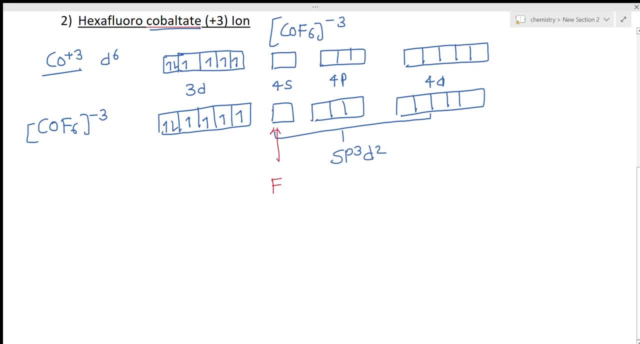 Then what will happen? These fluorines will donate a lone pair of electrons. here. These are the lone pair of electrons which are being donated by fluorine. These are the lone pair of electrons. So you can see that 6 lone pair of electrons are being donated by 6 fluorine ligands. 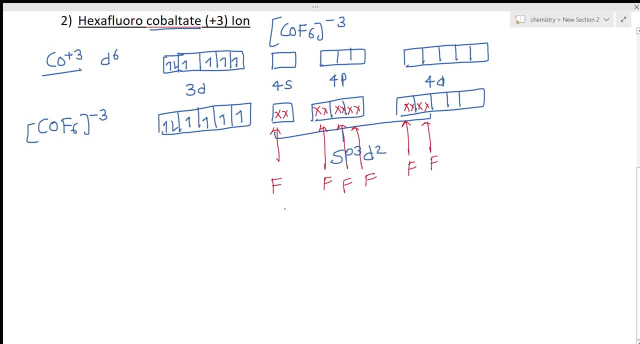 And in this way your COF6-3 complex is formed. Now look at this complex, These unpaired electrons In the free metal. how many were there? 4. Here, also 4 unpaired electrons are present. 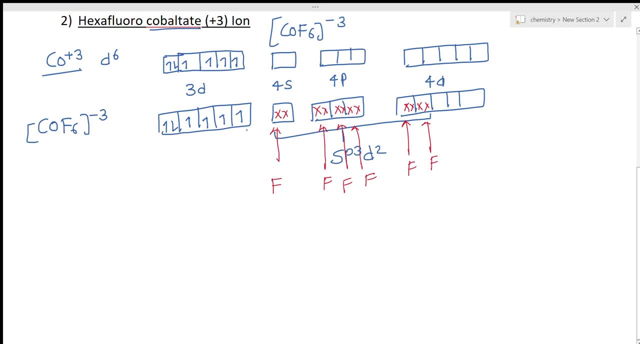 That is, the number of unpaired electrons has not decreased. Either it would have increased or remained the same. So what will we call such complexes? We will call them high spin complexes. So now, what is the complex that you are getting to see? 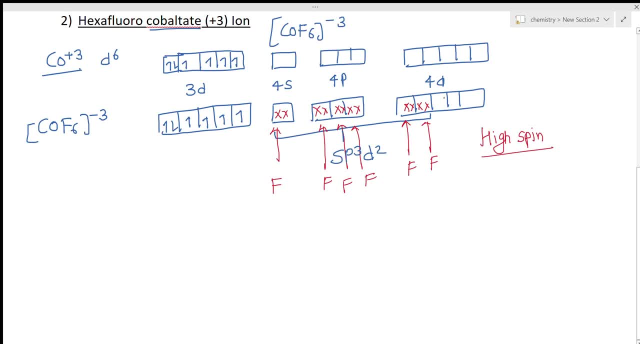 It is a high spin complex. Second thing: Here the outer d orbital is involved. You have seen that the outer d orbital is used. So what will we call such complexes? We will call them outer orbital complexes. So whenever outer orbital complexes are formed, 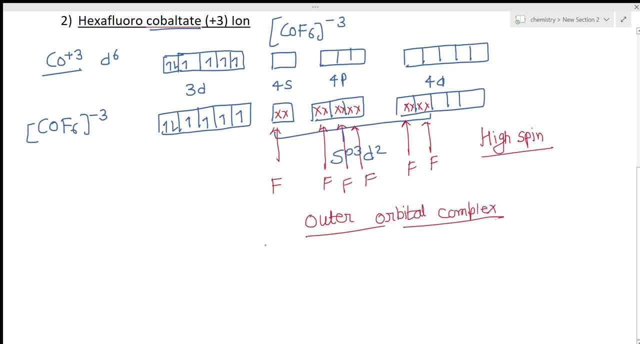 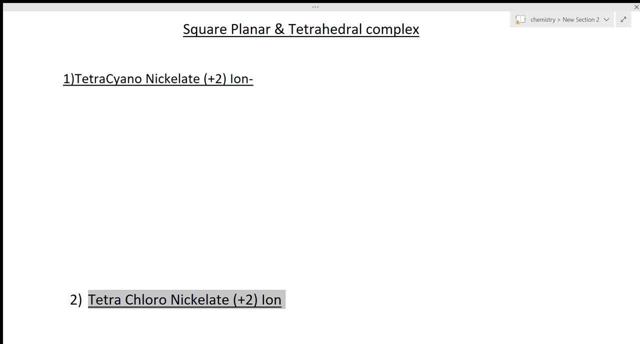 we get to see high spin complexes as a result of that. Let's see the next example. Now let's see square, planar and tetrahedral complexes. Whenever the coordination number of the complex is 4, there can be two types of geometries. 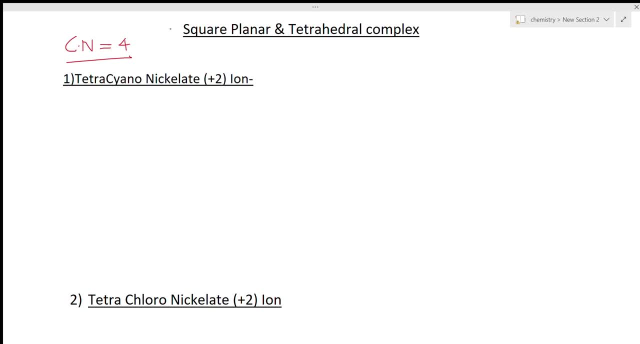 Either it can be a square planar or tetrahedral. Which one will it be? It depends on that metal and on its ligand. For example, you see tetra-sino-nickelate plus 2 ion. Here you have given NiCn4 minus 2.. 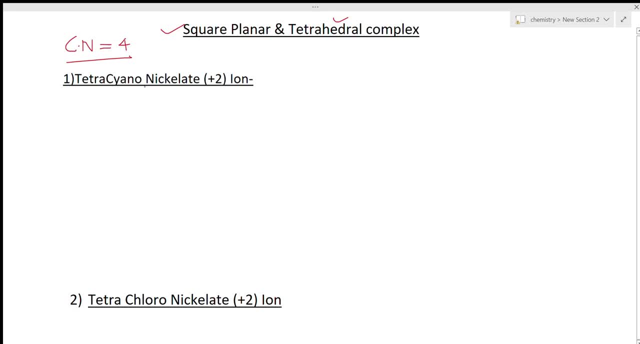 Okay, Here nickel is present in the plus 2 oxidation state. When nickel is present in the plus 2 oxidation state, it means that it is a D8 species. It is a D8 species. Okay, Let's see its configuration. 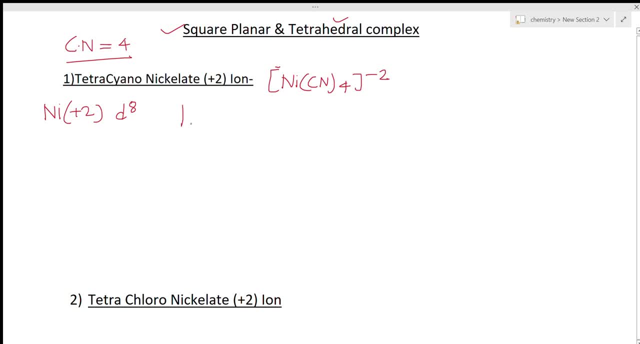 Here. this is your d orbital: 1,, 2,, 3,, 4,, 5,, 6,, 7, 8.. This is your 8 electrons. Here is S orbital and this is your P orbital. 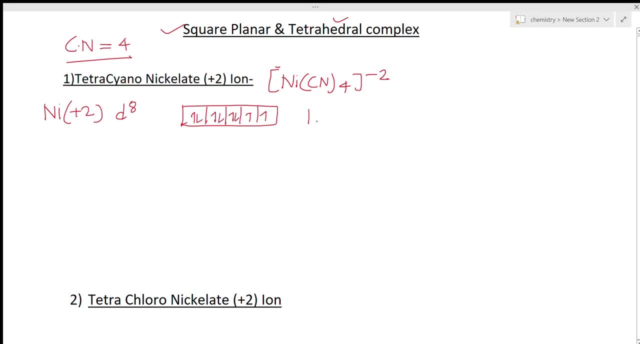 Okay, So here you can see: this is your 3d orbital, This is 4s and this is 4p. Now what did you see? first, That the coordination number is 4.. Here, 4 ligands are associated. 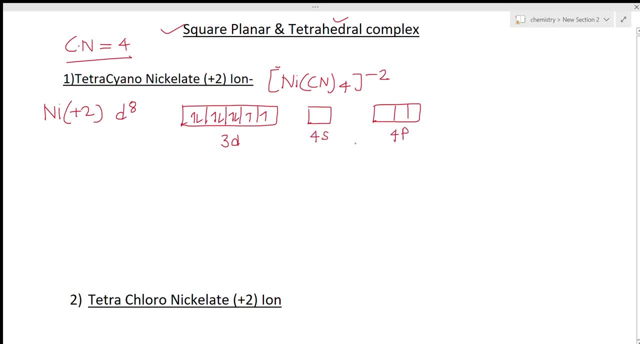 Means 4s is associated with 4.. So 4s is associated with 4.. Now you will see that the coordination number is 4.. Now you will see that the coordination number is 4.. which means it needs 4 empty orbitals. 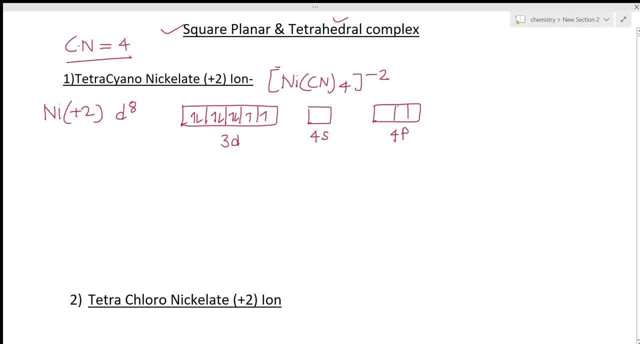 So where can these 4 empty orbitals come from? Either these 4s and 4p orbitals are involved. then there will be sp3 hybridization, Or what can happen When the electrons of d orbitals pair up. 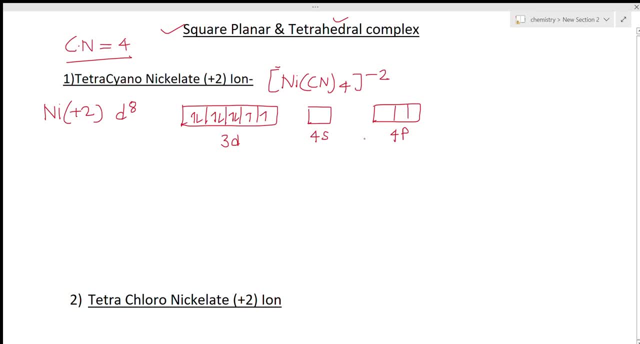 then 1d orbital can also be available and there can be sp2 hybridization. Both cases can happen. Actually, it depends on the ligand. Here the ligand given is cyanide ligand. So when cyanide ligand is present, 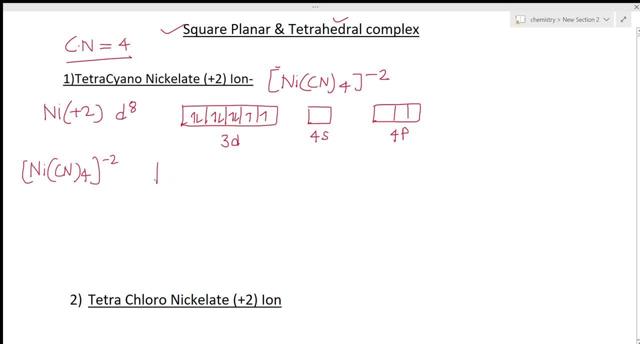 it is a strong field ligand. What is this? It is a strong field ligand. What will it do? It will pair the electrons, So these electrons will quickly pair up here. Now see what happened to d orbital. It is available. 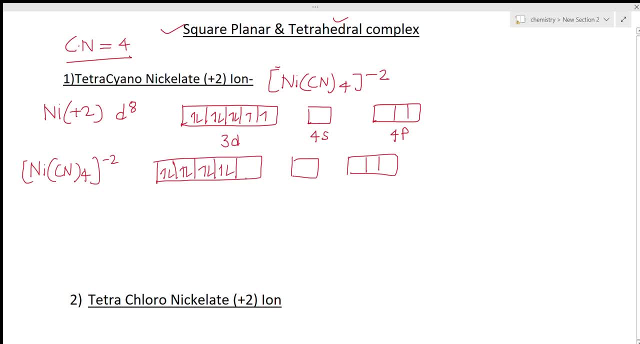 1d orbital is available here. So then 1,, 2,, 3 and 4.. 4 orbitals will participate in hybridization. So how will hybridization happen? There will be dsp2 hybridization. Due to this dsp2 hybridization, 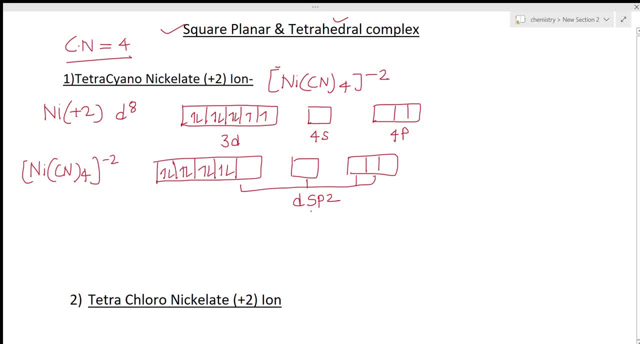 4 dsp2 hybrid orbitals will be formed. And whenever dsp2 hybridization happens, do you know what geometry is? Square planar? Square planar geometry is there. So these electrons will be given by cyanide ligand. These electrons will be filled in these orbitals. 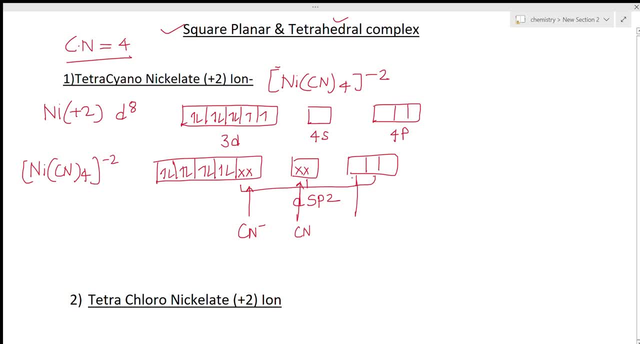 In this way, these electrons will be filled here And in this way your NiCN4-2 complex will be formed. You can see that all the electrons have been paired up here. So how is the complex being formed? It is a low spin complex. 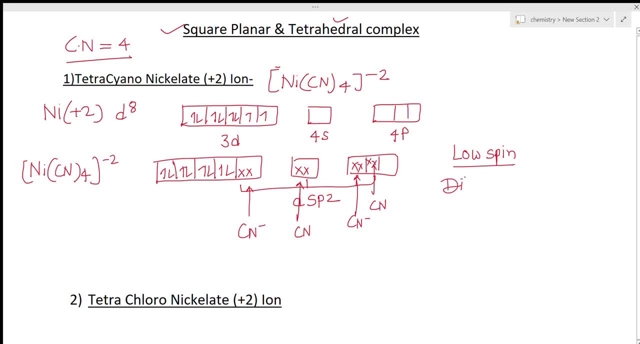 That is, there is no unpaired electron in the complex. So how is it? It is diamagnetic. How is hybridization in this? It is dsp2.. So how is its geometry? It is square planar, Okay. 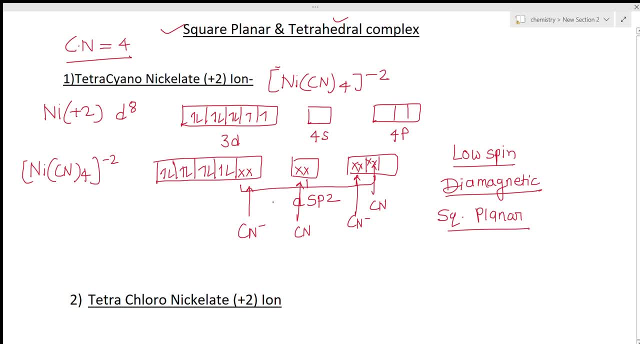 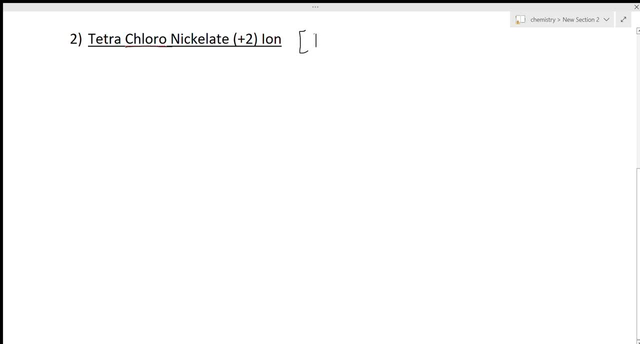 This is very clear. Many questions are asked on this, So remember this point specially Okay. The second example is your tetrachloronucleate plus 2 ion, NiCl4-2.. Okay, Here your nickel is in the plus 2 oxidation state. 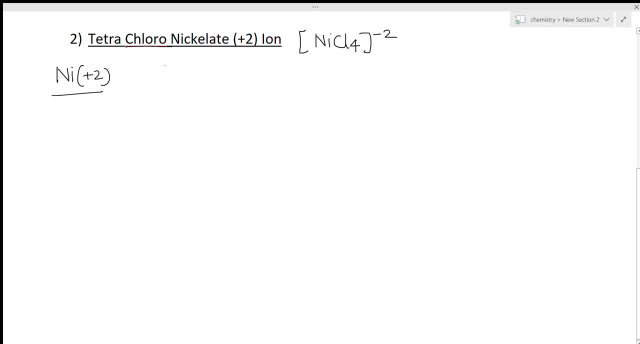 Again, it is in the plus 2 oxidation state. Okay, The same condition will be there: 1,, 2,, 3,, 4,, 5,, 6,, 7 and 8 electrons. Now see what happens here. 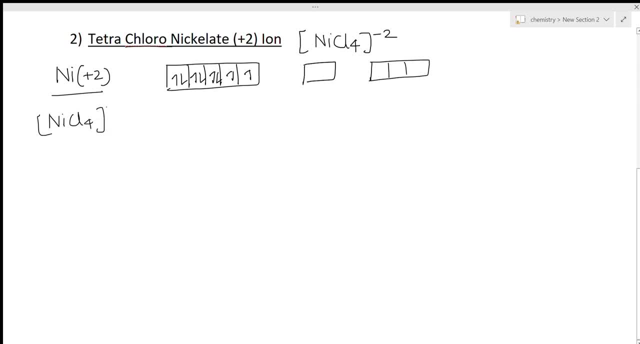 In this case, the serial ligand given to you. Actually, this serial ligand is a weak field ligand, So it cannot pair the electrons, So the electrons remain as it is here, That is, there is no pairing of these electrons.